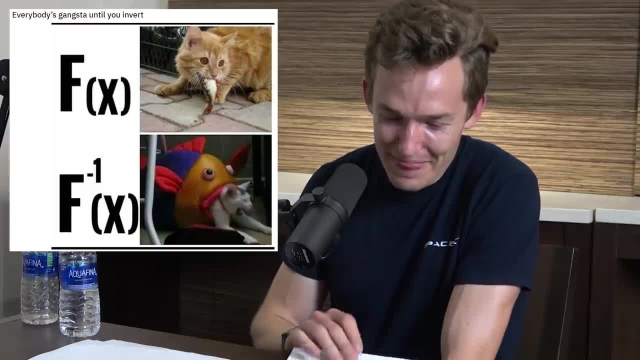 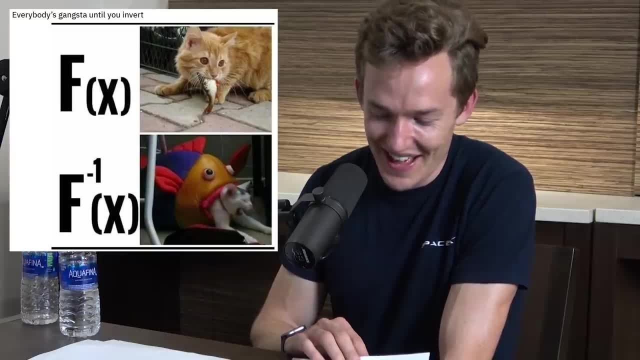 I think there's a. so what is that? I think that's a fish eating a cat. Yeah, no, so it's a cat eating a fish and then the fish eating the cat. So I just have to say A plus, This should be in every algebra textbook. That's my meme review. 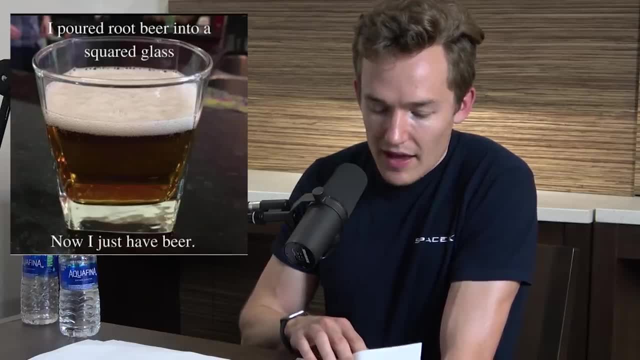 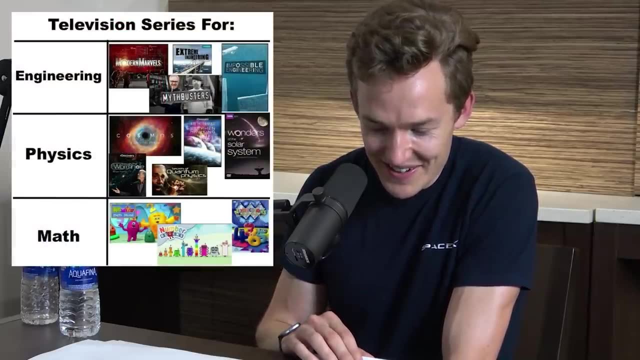 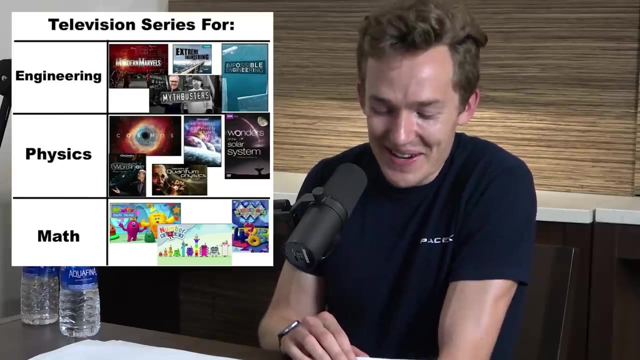 I poured root beer into a squared glass. Now I just have beer. Tired, Not impressed, Not impressed. Engineering Got Mythbusters and such Physics. Oh, this is a prior discussion. This is a prior discussion. No one thinks that you could popularize math. 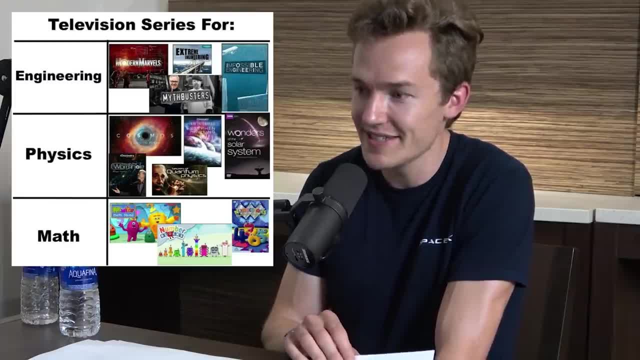 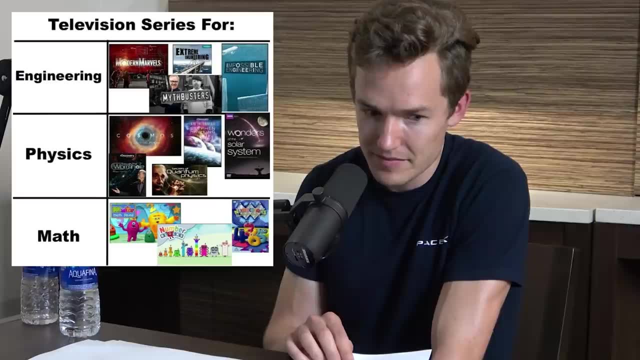 That's interesting, So it ends with that's. that is insightful, Poignant, So do you think it's? so do you think there's? it could be a cosmos for mathematics? Yeah, I actually. i think there's huge appetite for it. i think numberphile proves this fact, and, and your chair. 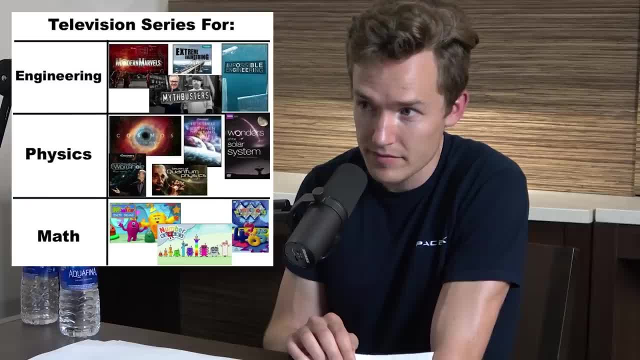 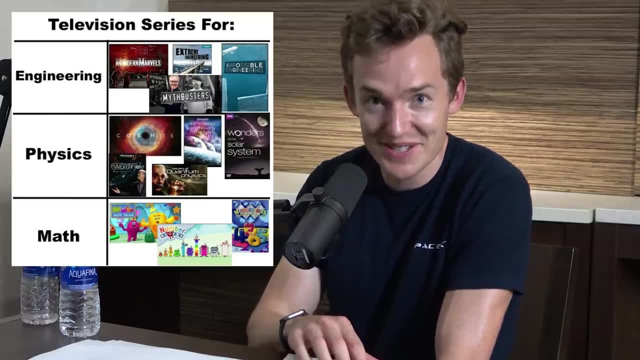 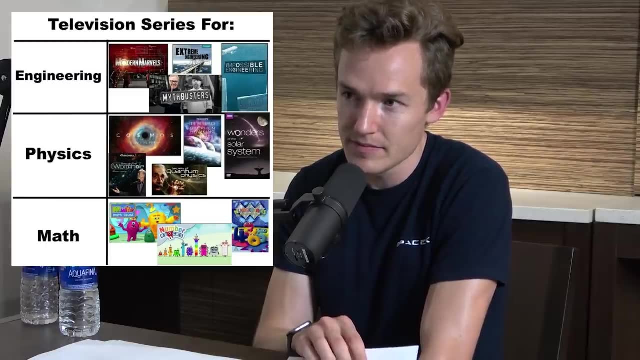 i mean that's true, but there's not for some reason. do you think there'll be a netflix show one day with? uh, anyone at netflix is watching this. i will host it for you, you just call me. but do you think you could have um like a general public kind of show like osmos and do math 100? i, i think it. 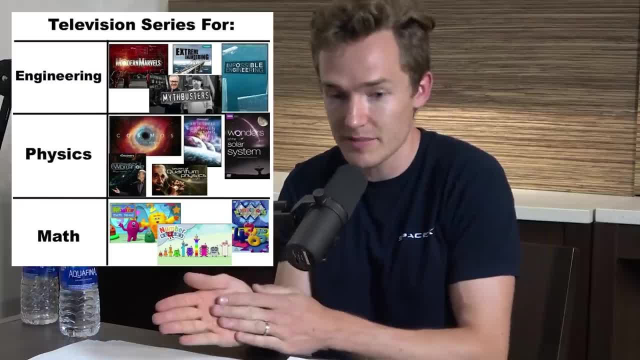 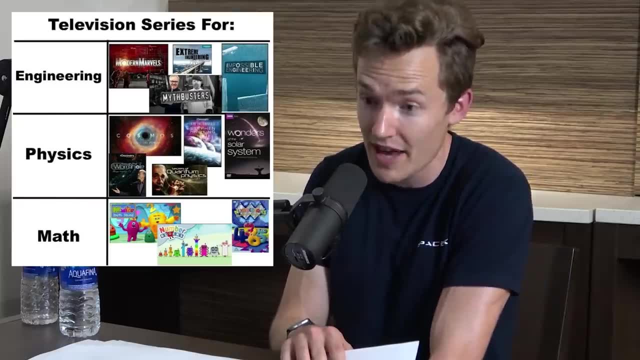 wouldn't be easy. um, because you know you've got this tight line between: are you doing it substantively or you're just waving your hands. i think there's enough really interesting math that you can substantively get across, and i do think there's a pretty big appetite for it. um, 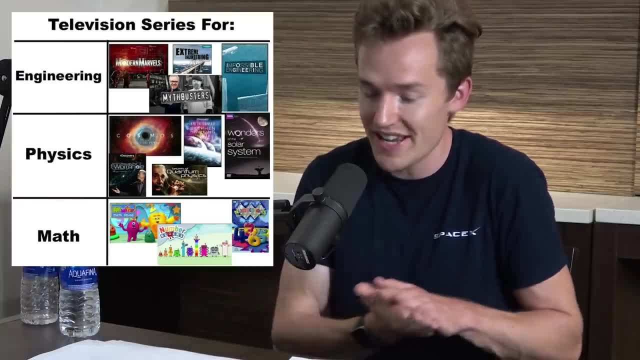 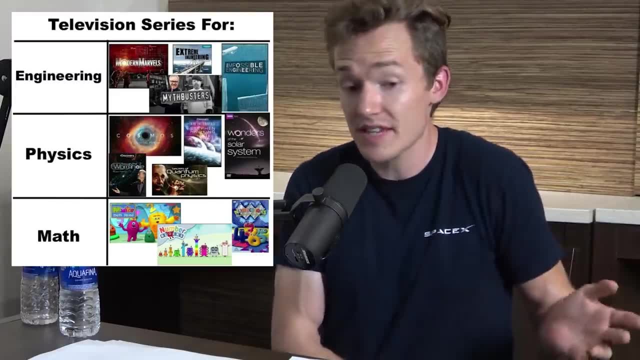 the reason i say numberphile isn't just that numberphile is great, but that brady has like 10 projects of very similarly styled channels and numberphile is the biggest among them by far. but they're all successful. they're all successful, but i would have guessed if you were just pitching. 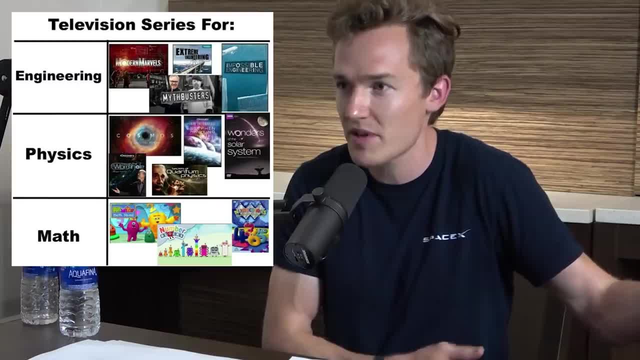 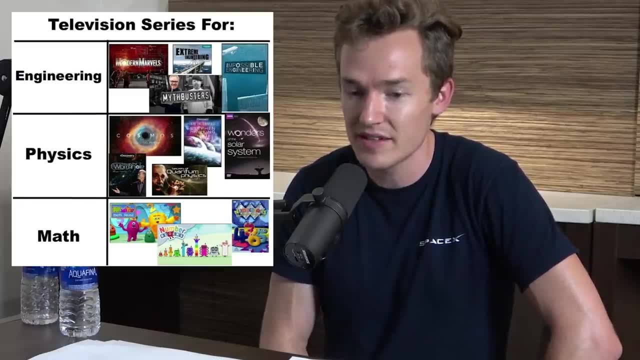 these products, you know, like 10 years ago, like, oh, the channel on physics will be very popular, the chemistry one will be pretty popular, the numbers one- i don't know some people that might be like third or something, but the idea that the one about math is the most popular of his channels by far. 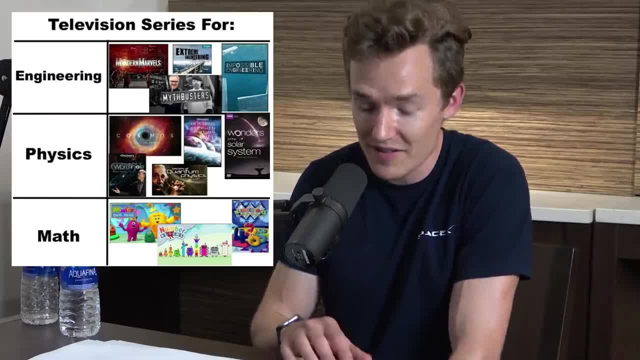 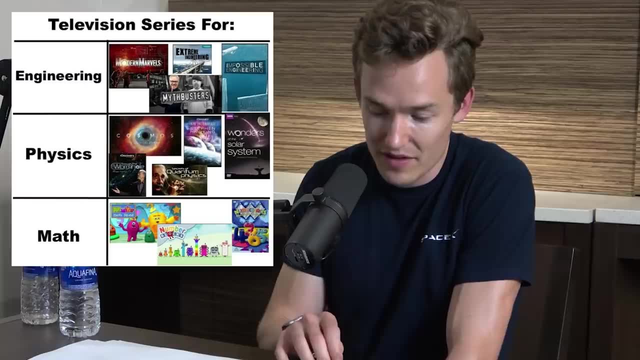 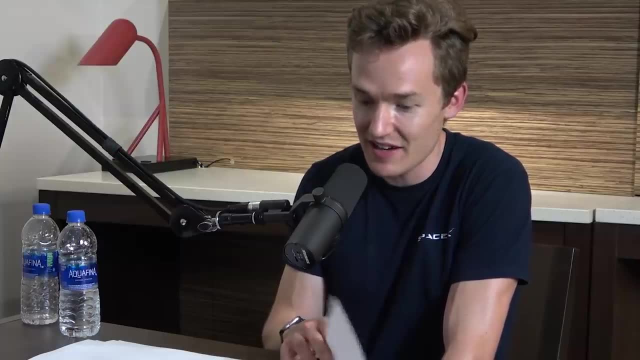 even though they're similar styles. i does, i, i does, i do think speaks to the fact that there is a unsatiated appetite for real, a real understanding of what gets mathematicians going. and, uh, i think a netflix type entity might recognize that. you heard it here, netflix.